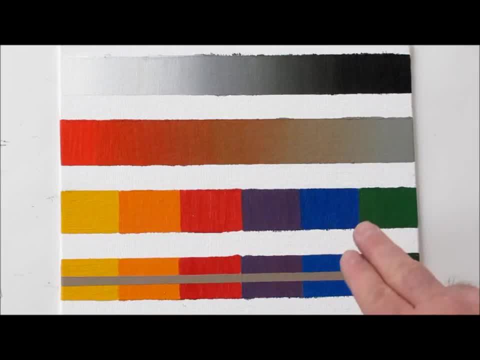 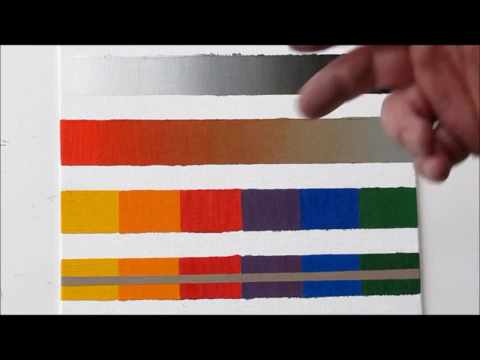 Is it part of the yellow family, the orange, the red, violet, blue or green? So the three characteristics of color once again are your value, your intensity and your hue. Again, your color families. This last one shows again our color families. 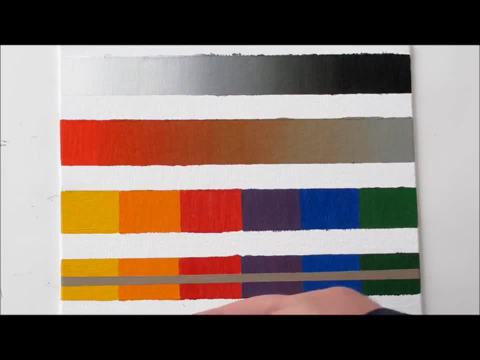 And it shows a gray stripe. This just shows how gray can shift depending on what color it is placed next to. So this really has. we can just kind of ignore that. I'm just explaining why it's here. But so the three again, the three characteristics are our value, our intensity and our hue. 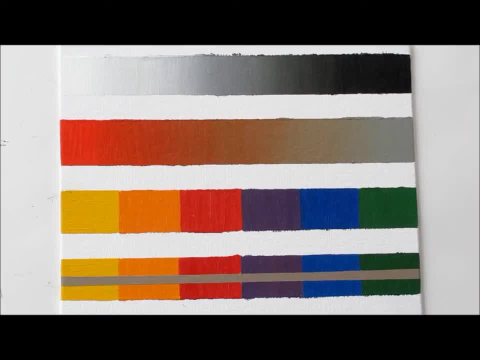 This has been Kevin McCain, with Kevin McCain Studios. Find out more about my painting workshops. Find out more about my artwork. I'll see you next time. Check out the illustrations I've done over my career at kevinmccainstudioscom. Thank, you so much. Have a good day. 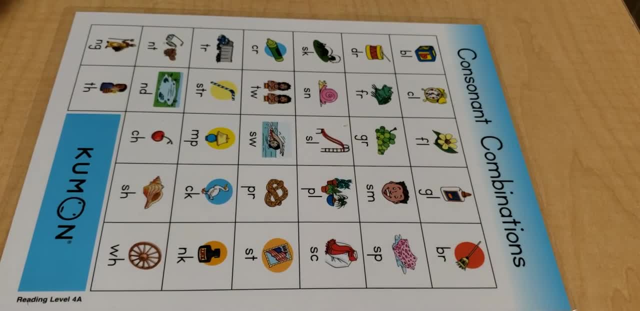 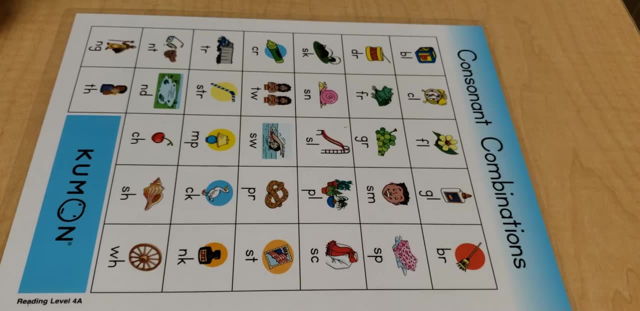 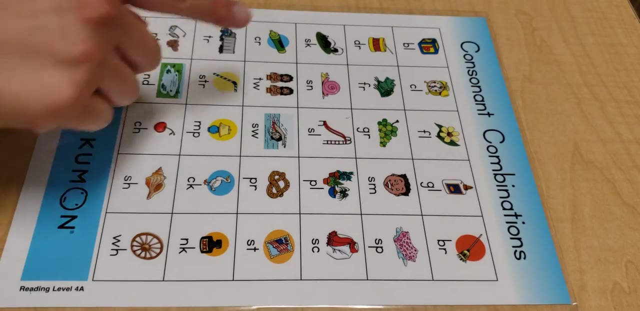 This is an instructional video on how to do the consonant combinations chart with your child at home. Make sure that your child says the sound together and not separately, while pointing at the sound at the bottom. Then say the name of the picture on top: Bull block, Cool clock, Full flower. 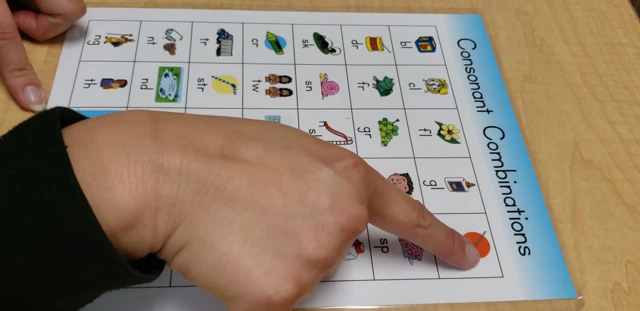 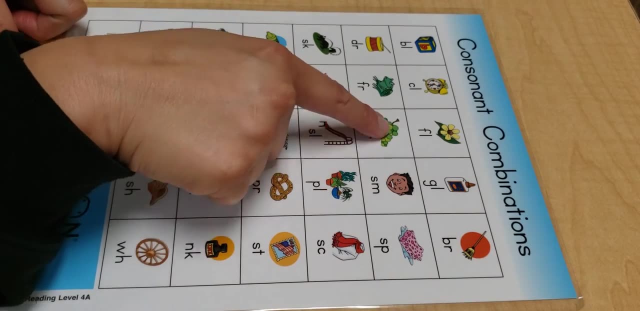 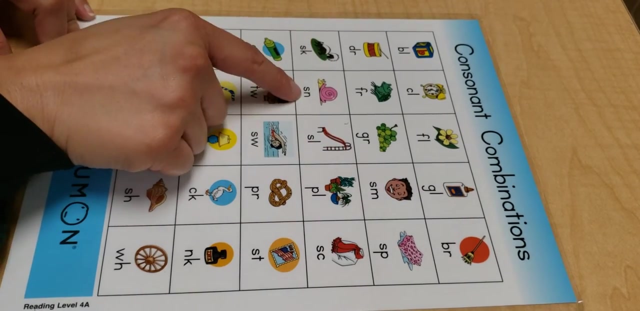 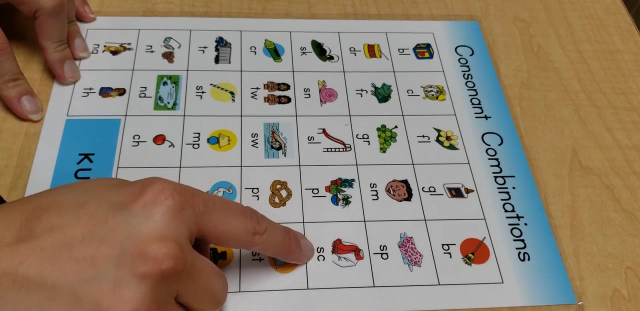 Glue, glue, Brr broom, Drr drum, Frr frog, Grr grapes Sm smile Sp sponge Sk skunk Sn snail, Sl slide Pull, lance Sk scarf, Krr crayon. 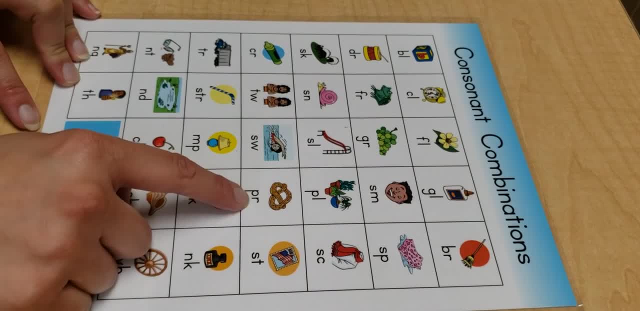 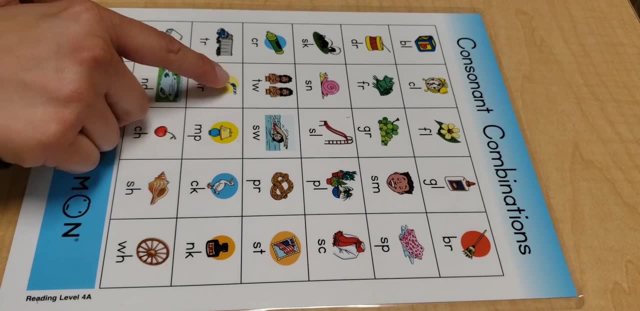 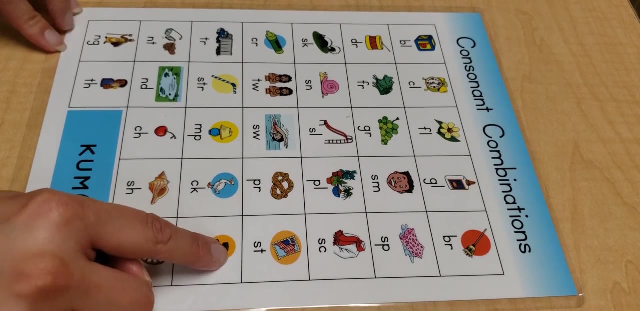 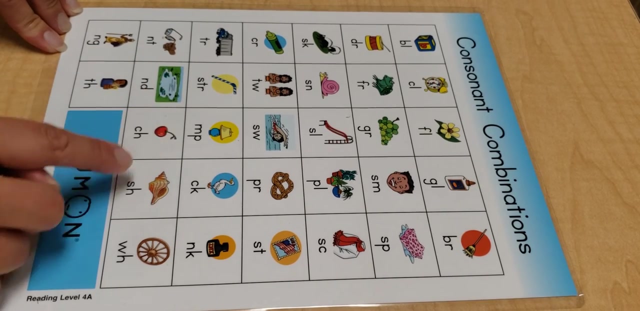 Twr twr Twints Sw swim Prr pretzel St stamp Ter truck Str straw Mp lamp K duck Nk ink Nt bent Nd pond Ch cherry Sh shell W wheel N.